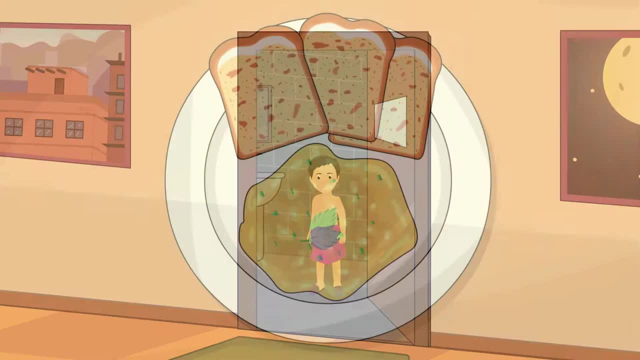 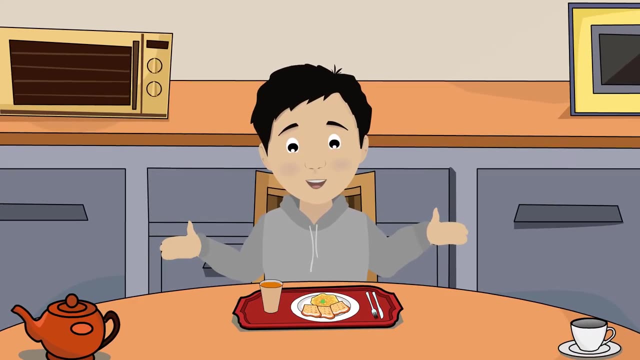 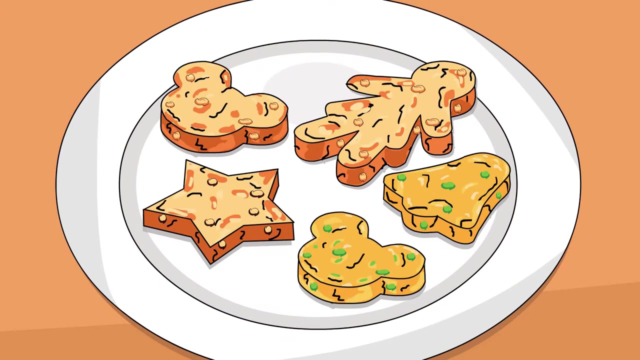 He let out a sigh and opened the door. An omelette with toast and orange juice had been set out for his breakfast. Got to make this interesting, he thought, and pulled out a set of cookie cutters. He cut out some shapes and while he was admiring them, the school van was heard honking outside. 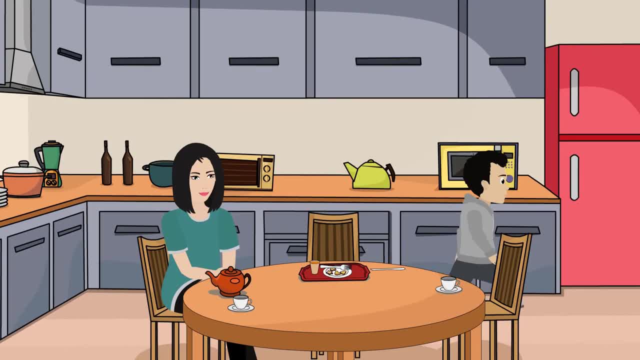 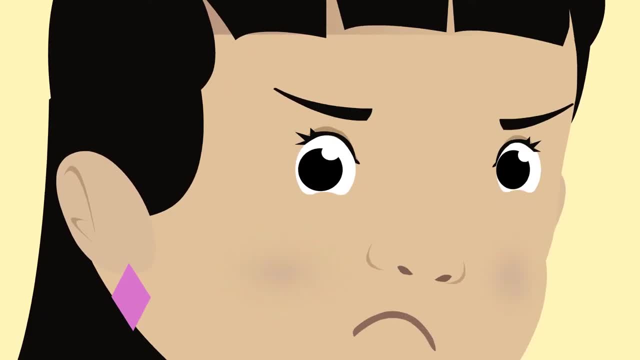 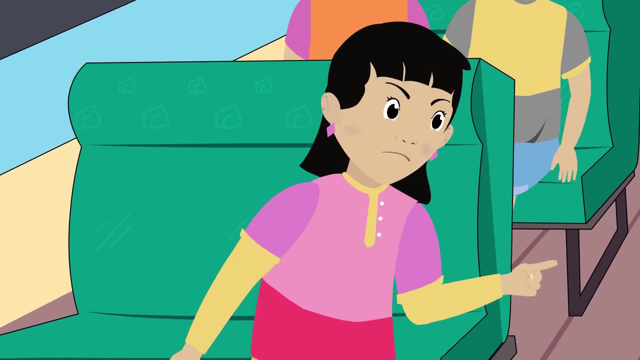 Oh no, he muttered. no time to eat now. And just when he was about to leave, he remembered that his bag was still in his room. Oh boy, he got some really dirty looks when he got on the van. You better not get late. punishment because of you, cried out a pesky girl. 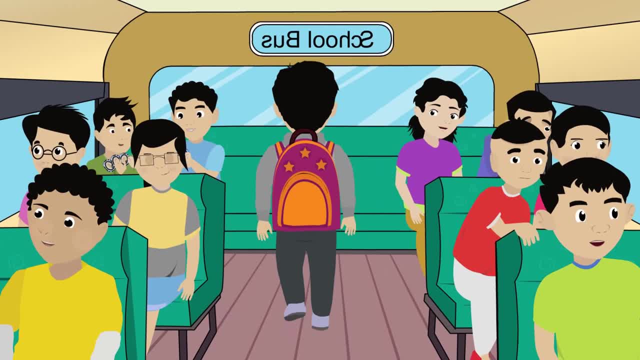 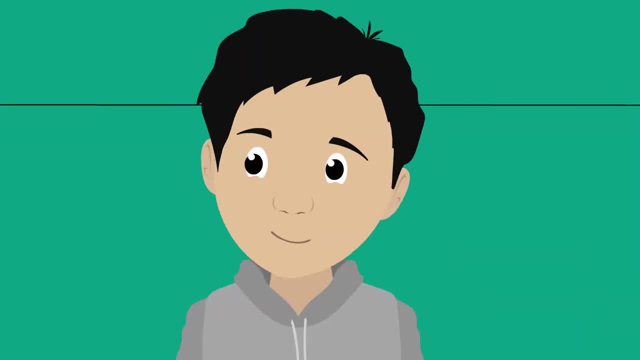 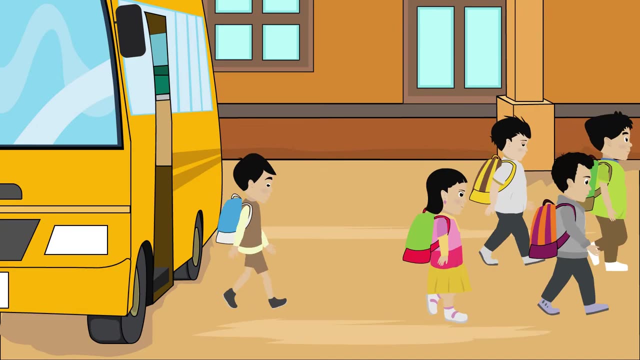 Ankit just made a face. He looked at her and went right back to sit with his friends. They were sharing their latest cricket cards that they had collected. He had left his at home in all that hurry. When he entered his class that day he was surprised to see jars on everyone's table. 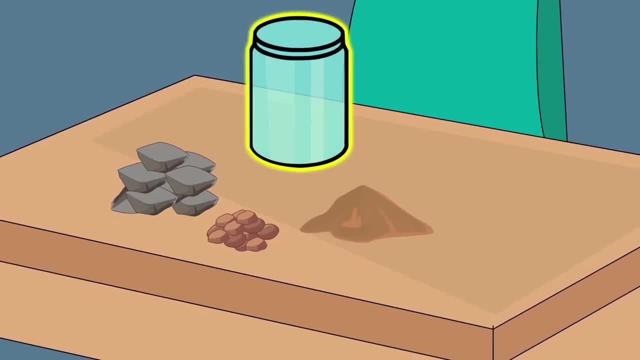 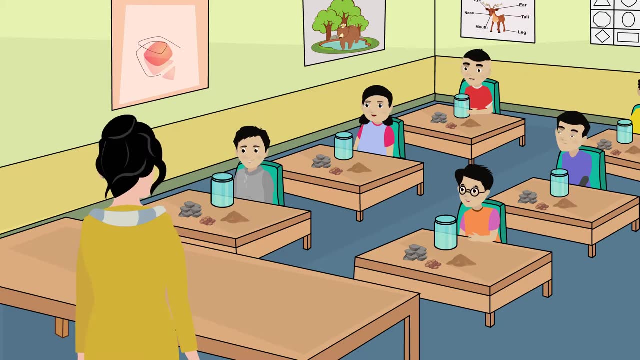 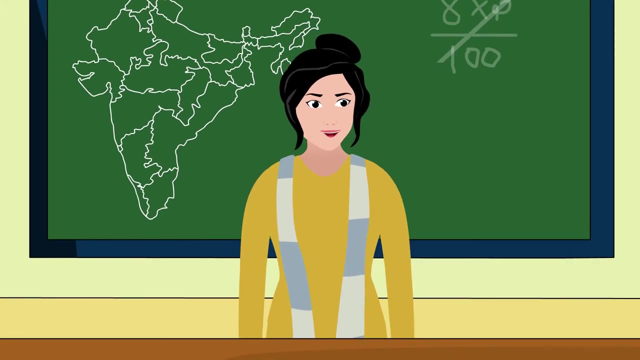 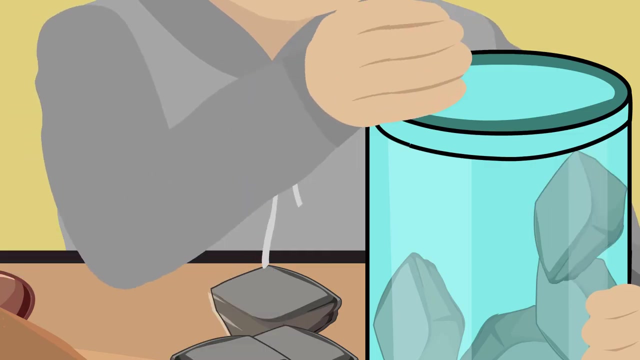 Rocks and small stones had also been kept with the jar and sand. Their teacher welcomed them And explained that now that they knew how to read time, the next important part was to understand how best to use their time. She told them to remove the jar's lid and place as many rocks as they could. 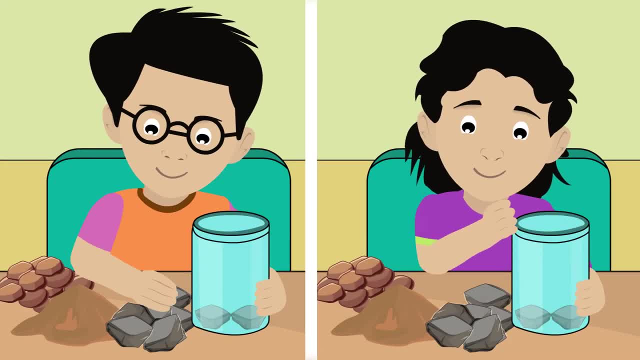 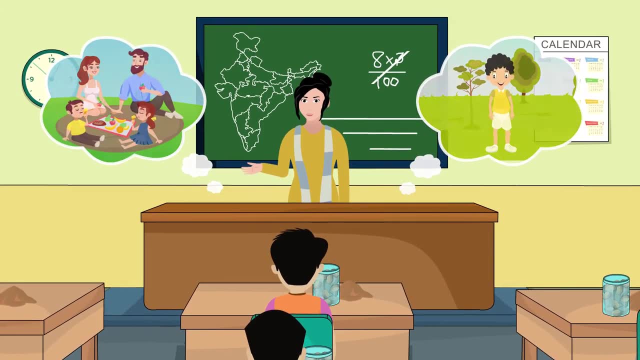 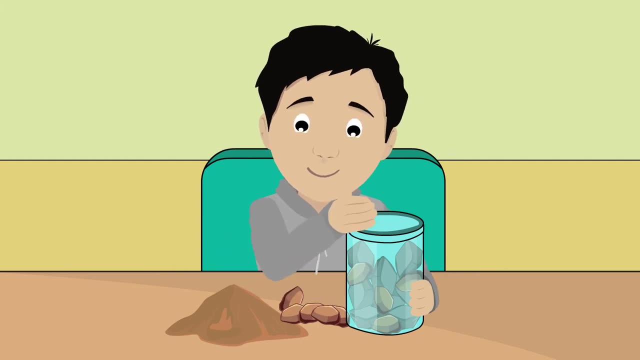 These rocks stand for all the important stuff They are a must to do, like your homework, exercise, spending family time, etc. Now she asked them to add as many small stones as they could. They all settled into the space between the rocks. 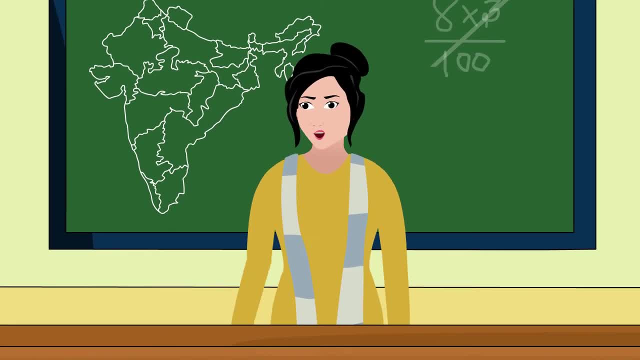 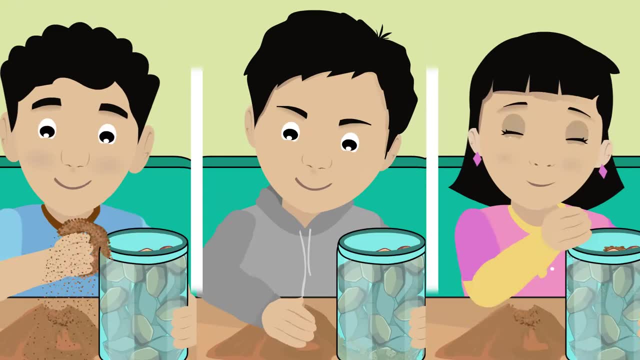 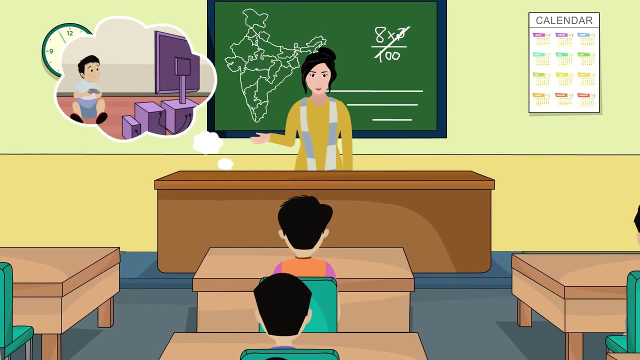 The stones are the things that are needed as extra skills, But not as important as the rocks, like tennis class, music lessons, etc. Lastly, they added sand, which she said stood for chill out things for them, like playing video games, watching TV, anything. 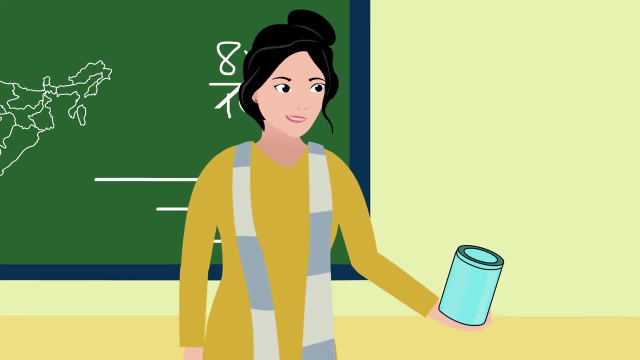 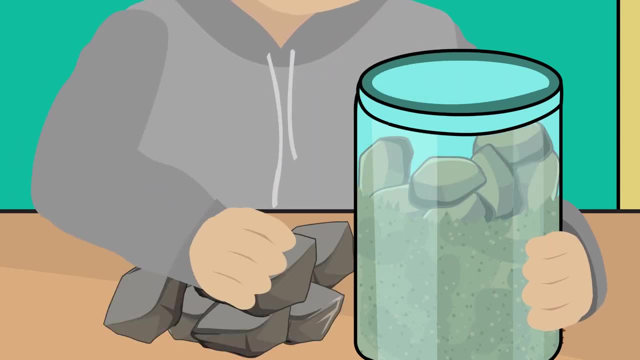 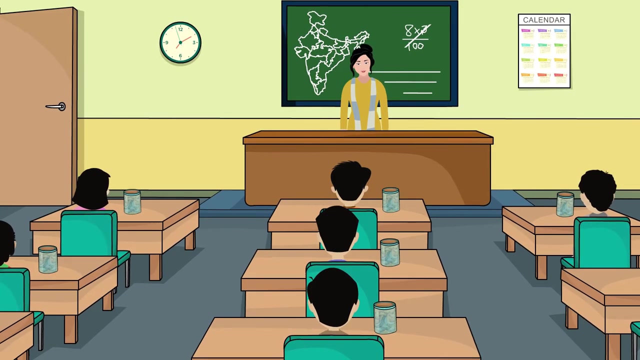 Anything that they loved doing, just to relax. Next she gave them another jar and asked them to put in the sand first, then the stones and lastly the rocks, But this time all the rocks would not fit. She told them that if their day was filled with the lesser important things, there would.